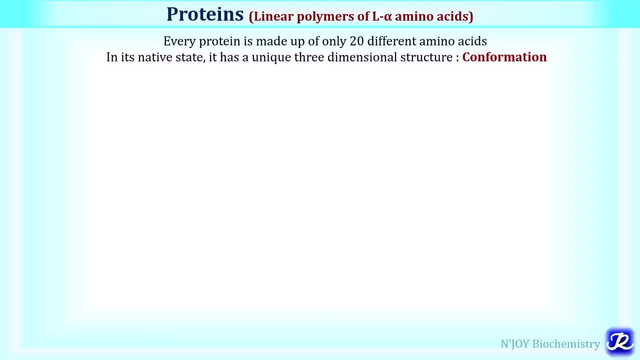 of only 20 different amino acids and the protein in its native state has a unique three-dimensional structure that is called as conformation. There is often confusion between two terms: configuration and conformation. So let's understand. Configuration is geometric relationship between a given set of atoms, For example L and D amino acid. this is the 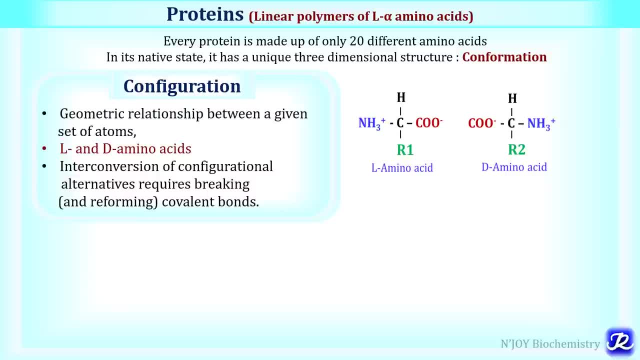 configuration. The interconversion of configurational alternatives requires breaking and reforming of covalent bonds. So this is L amino acid and D amino acid. this is the configuration. Conformation is special relationship of every atom in a molecule. An interconversion between: 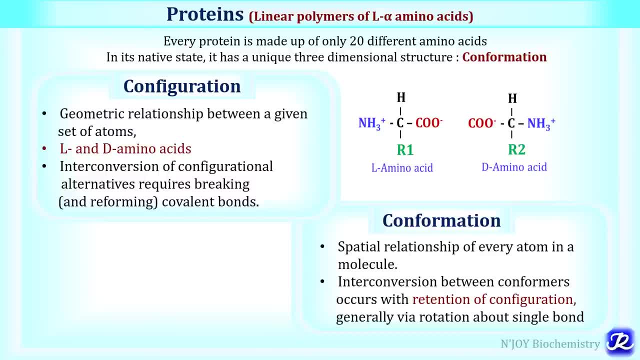 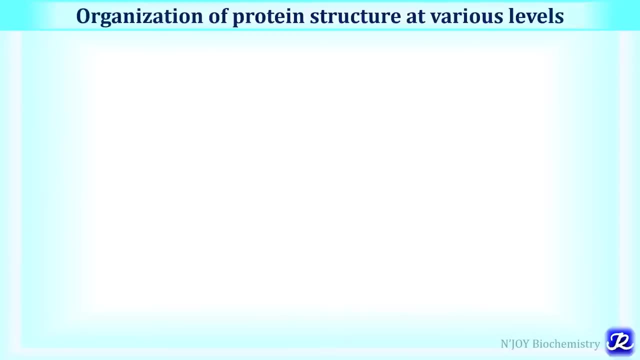 conformers occur with the retention of configuration and generally via rotation about single bonds, So there is no need of breaking and reforming covalent bonds in case of conformation. There are four levels of organization of protein structures Due to assembly of amino acids. 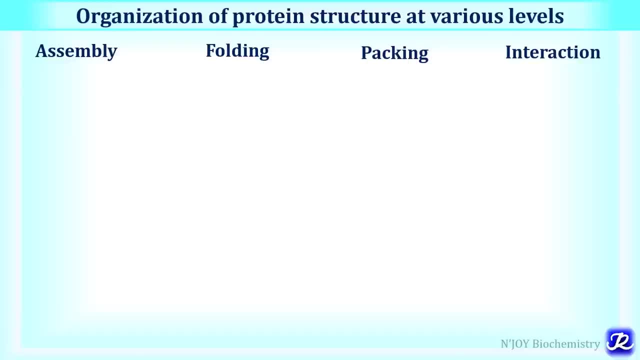 which are linked together by peptide bonds. then folding of that polypeptide chain, packing of that polypeptide chain and then interaction of different polypeptide chains. So all these four mechanisms- assembly, folding, packing and interaction- it leads to formation of four levels of organization of protein structure, that is, 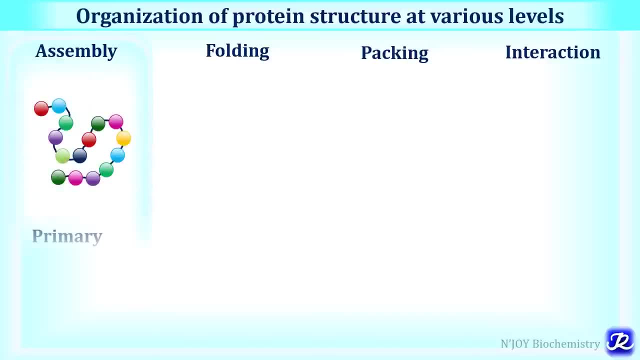 primary, secondary, tertiary and quaternary. So in the primary structure that is due to assembly of different amino acids. when the amino acids are linked together by peptide bonds, it results in the primary structure of protein. And when the primary structure leads to formation of polypeptide chain, when this polypeptide chain is folded. 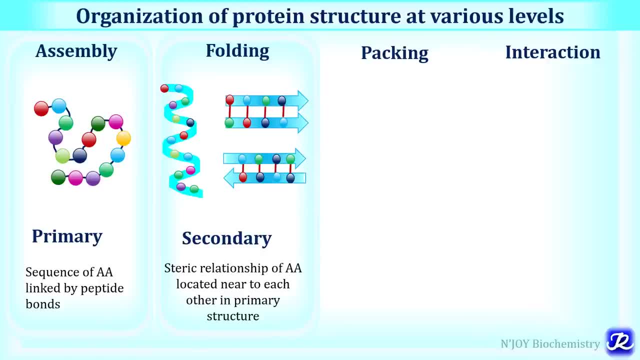 due to intermolecular hydrogen bonding. it results in the secondary structure and in this secondary structure there is steric relationship of amino acid located near to each other in the primary structure. So folding of primary structure results in the secondary structure. Now packing of that. 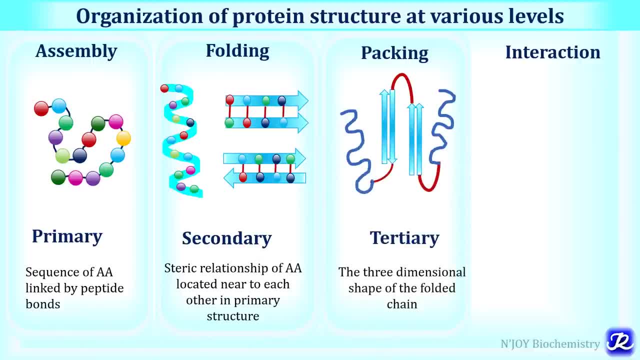 folded structure. in the three-dimensional structure it results in the secondary structure. So in the three-dimensional shape it is called as tertiary structure. So tertiary structure is nothing but the three-dimensional shape of the folded chain. Then comes interaction of different 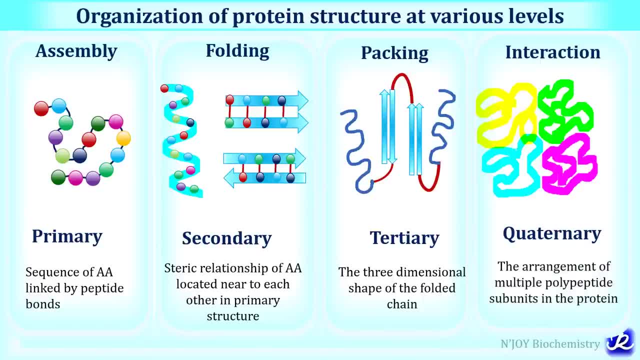 folded chains or polypeptide chain, So the arrangement of multiple polypeptide subunits in a protein. it is called as quaternary structure. So there are four levels of organization of protein structure: primary, secondary, tertiary and quaternary. 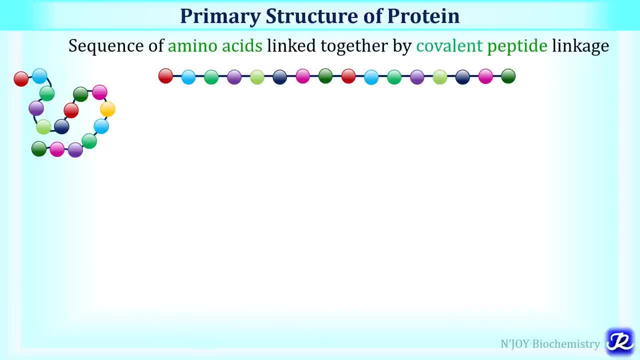 Let's first see the primary structure of protein. It is the sequence of amino acids linked together by covalent peptide linkage, So all the amino acids in this primary structure of protein. they are linked by peptide bond and this peptide bond is formed by two amino acids, So when one amino acid, it is linked with the other amino acid. 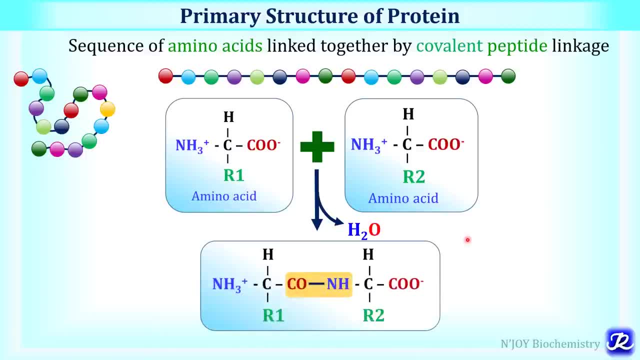 with the release of water molecule, there is formation of peptide bond. So how this peptide bond is formed? It is formed by amide linkage between alpha carboxyl group of amino acids and alpha carboxyl group of amino acids. So this is the alpha carboxyl group of one amino acid to the 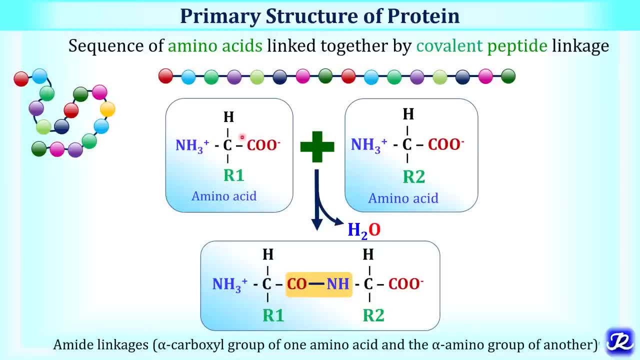 alpha amino group of another amino acid, So alpha carboxyl group of this amino acid number one. it condenses with alpha amino group of second amino acid. So there is release of one water molecule and there is formation of peptide bond. So this CONH, it is called as peptide bond, and 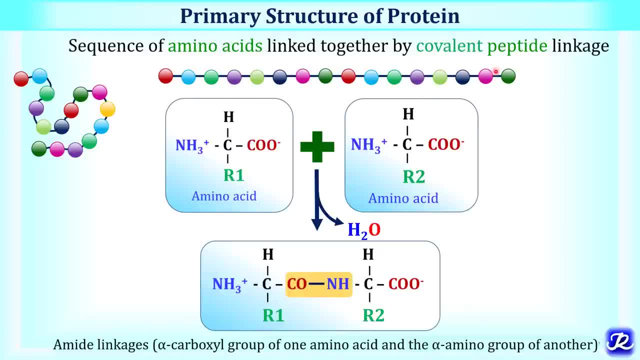 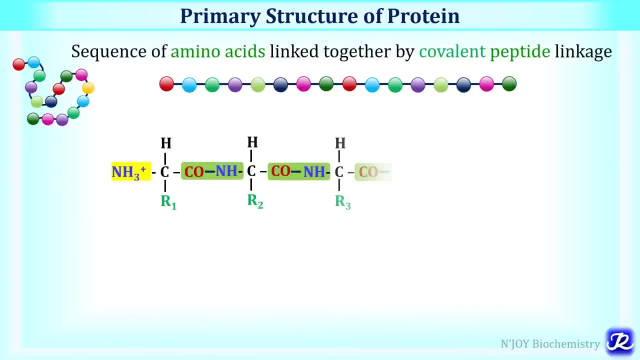 all the amino acids in a primary structure of protein. they are linked together by such peptide linkages. So the linkages of many amino acids through peptide bonds results in an unbranched chain called as polypeptide, and each amino acid in a polypeptide it is called as a residue or moiety. 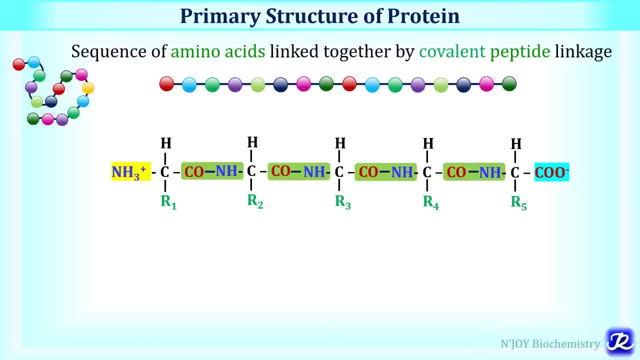 and each polypeptide. it is having free amino group at one end, and it is called as amino terminal or end terminal, and it has free carboxylic group at the other end, and it is called as carboxy terminal or C terminal. 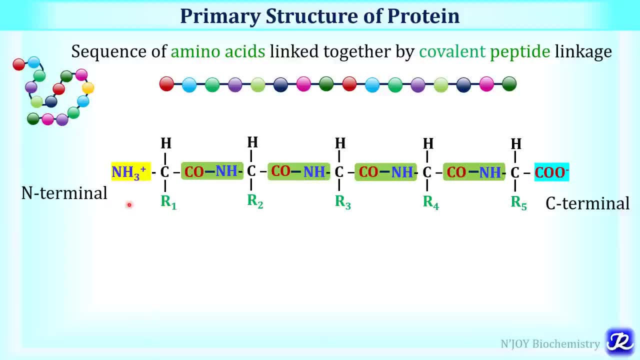 And the amino acid which is contributing to this amino terminal. it is the first amino acid and the amino acid which is contributing to the carboxy terminal. it is the last amino acid and usually this N terminal amino acid. it is written on the left hand side when the sequence of protein is: 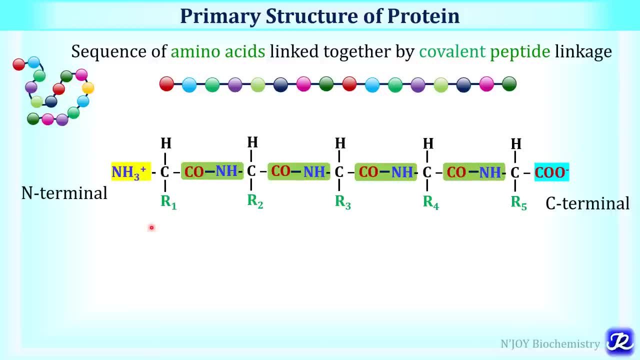 denoted. Also, the biosynthesis of amino acid starts from the amino terminal N, So the primary structure of protein is nothing but linear sequence of amino acids held together by peptide bonds. It is the backbone of protein and it is responsible for the function of protein. Each 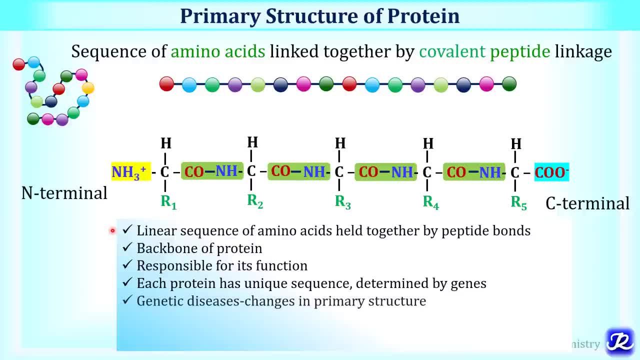 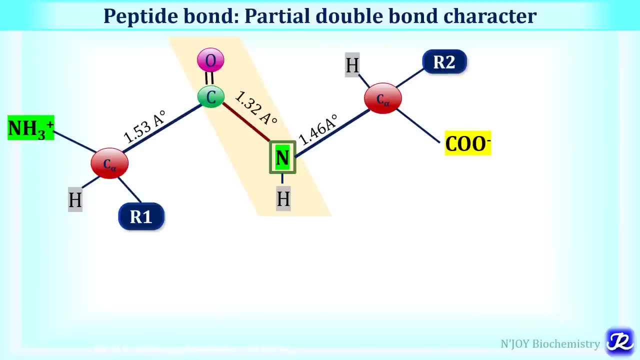 protein has unique sequence which is determined by genes, and any change in the primary structure leads to genetic disease. and three-dimensional structure of a protein. it is determined by its amino acid sequence. The peptide bond of primary structure of protein has partial double bond character. This is schematic representation of a peptide bond which is formed between the: 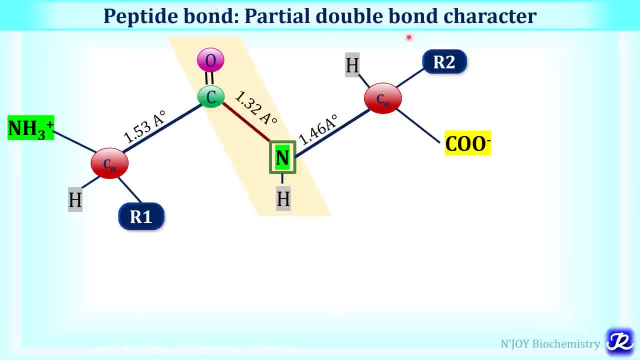 two amino acids. this is the first amino acid and this is the second amino acid. Between the Cα of one amino acid and the Cα of adjacent amino acid, there are three bonds are present. The first bond is between Cα of one amino acid and this carbon, and second bond is between C and N. and third bond is between: 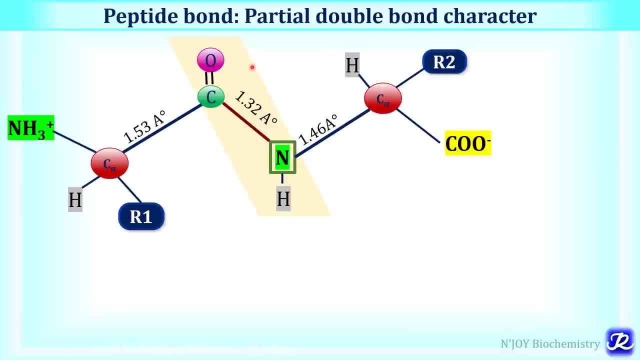 Cα of second amino acid and this N. So the peptide bond, it is called as partial. it has partial double bond character because the carbonyl oxygen, this carbonyl oxygen, it has a partial negative charge and amide nitrogen has a partial positive charge and that's why it is called as it has partial. 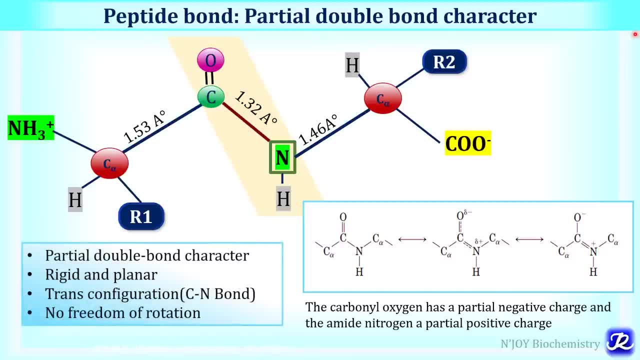 double bond character and because of this partial double bond character there is no freedom of rotation around this peptide bond. There is trans configuration of oxygen and hydrogen atom in this peptide bond and it is rigid and planar. But rotation is possible around this bond. that is the bond between Cα and C and Cα and N, So the rotation between Cα and N. it is called as: 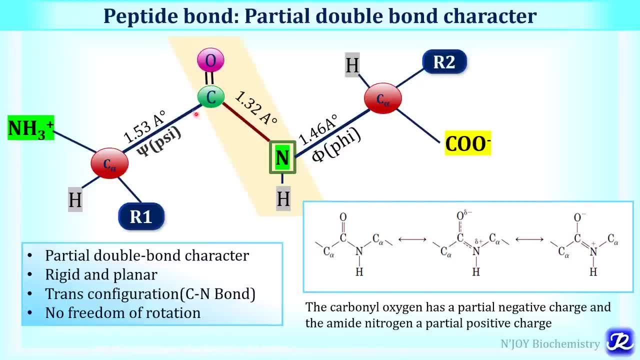 the angle is called as Φ and the angle of rotation between Cα and C it is called as Ψ. So there is freedom of rotation between this Φ and Ψ angle, but there is no freedom of rotation around this CN. that is the peptide bond, because this bond has partial double bond character. Now the second level. 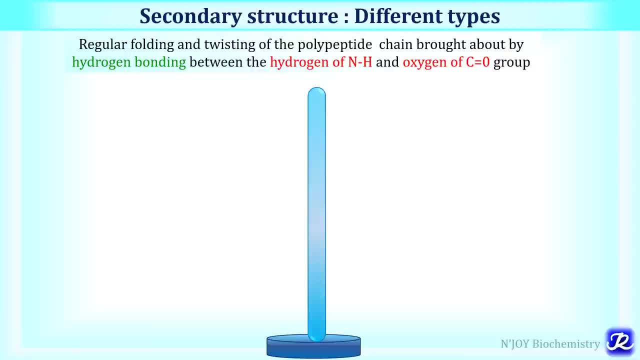 of organization is secondary structures, and there are different types of secondary structure. and these secondary structures are formed by regular folding and twisting of polypeptide chain which is brought about by hydrogen bonding between hydrogen of NH and oxygen of CO group. So there are various types of secondary structure. The first and most common is α, helix. second is β. 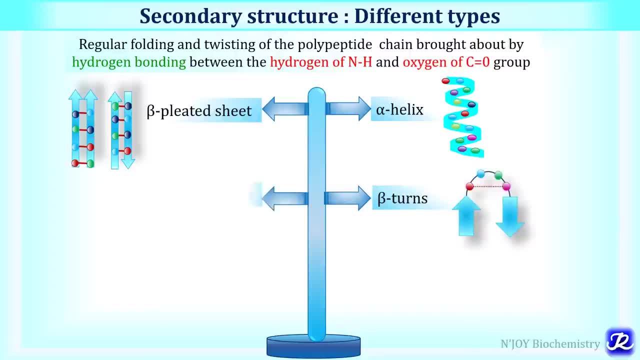 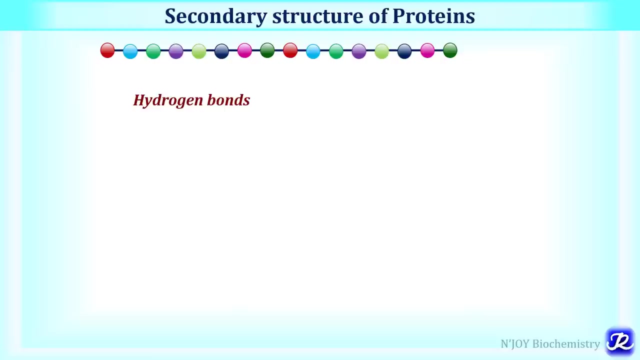 pleated sheet, then β turns, There are loops and bends, There are various super secondary structures and triple helix. So these are the various secondary structures that can be found in protein structure. Secondary structure of protein results from the folding of a primary structure of protein due to formation of intramolecular hydrogen. 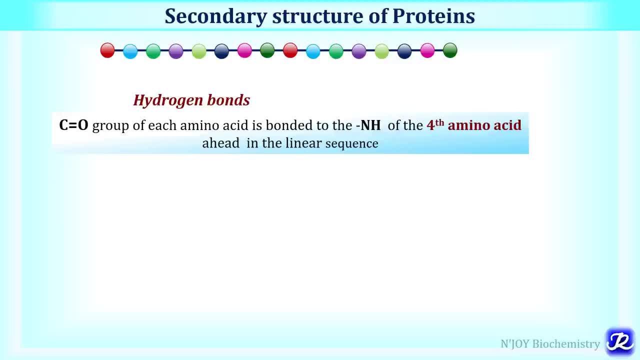 bonding and this hydrogen bonds are formed by CO group of each amino acid when it is bonded to NH of the fourth amino acid ahead in the linear structure í. So this hydrogen bonding, intramolecular hydrogen bonding, is formed between the CO group of 1 amino acid. 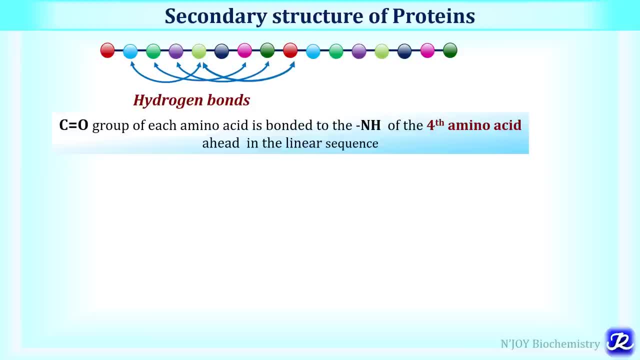 and it is bound to fourth amino acid ahead in the linear sequence and it results in the folding of primary structure of protein that forms the secondary structure of protein. Here you can see in this picture, there is hydrogen bond that is formed between the CO of doubling of the Lewis as well as itsеты, the predominant 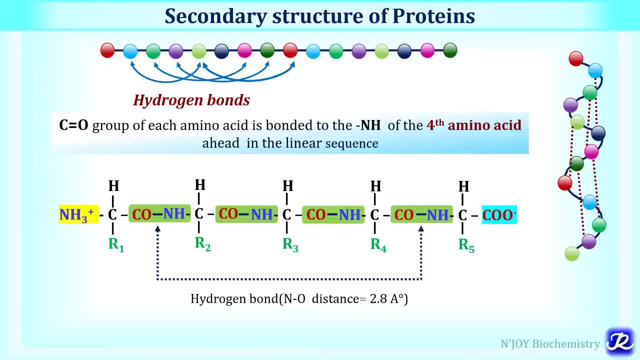 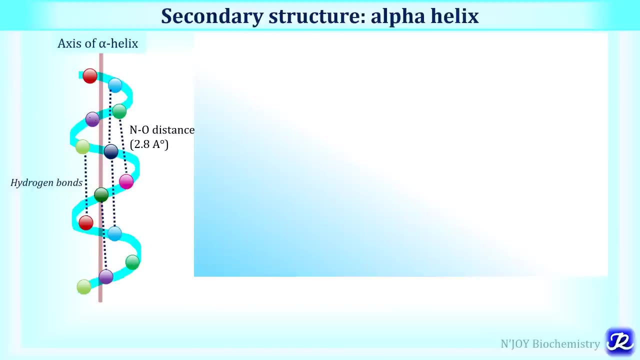 of one amino acid to the NH of fourth amino acid and the distance between this NO distance is 2.8 Armstrong unit. So the secondary structure of protein is formed by folding of primary structure due to intramolecular hydrogen bonding. So there are various types of secondary structures and the 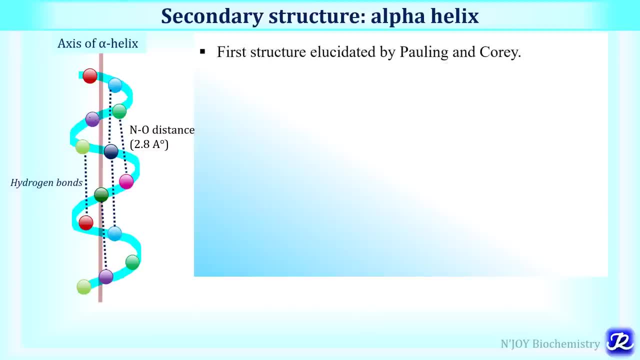 first one is alpha helix. It is called as alpha because it is the first structure elucidated by scientists Pauling and Corey. It is the most common and stable conformation which is formed spontaneously with the lowest energy and because of intramolecular hydrogen bonding, the primary 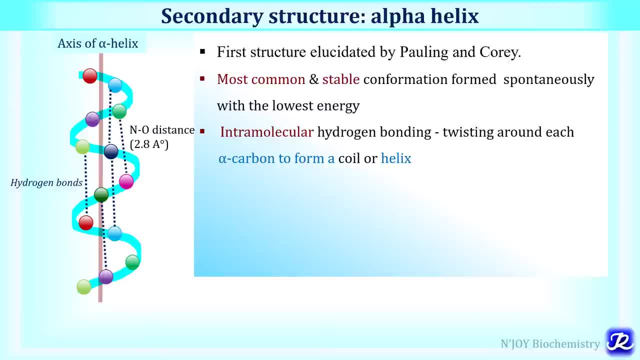 structure. it is twisted around alpha carbon to form a coil, or it is called as helix. It is a helical structure. and this helical structure, it is stabilized by hydrogen bonds. and this coil structure, it is a tightly coiled polypeptide backbone. it has 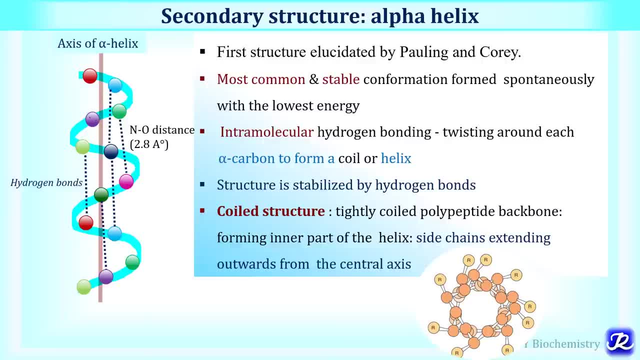 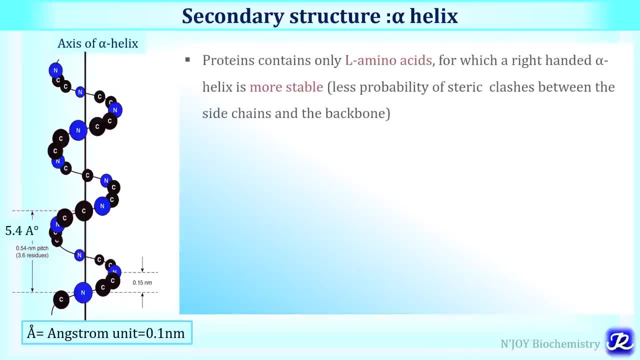 a helical structure and it is stabilized by hydrogen bonds and this coil structure. it is a helical structure which forms inner part of the helix and there are side chains which are extending outwards from the central axis. Protein contains only L alpha amino acid and for which a right-handed 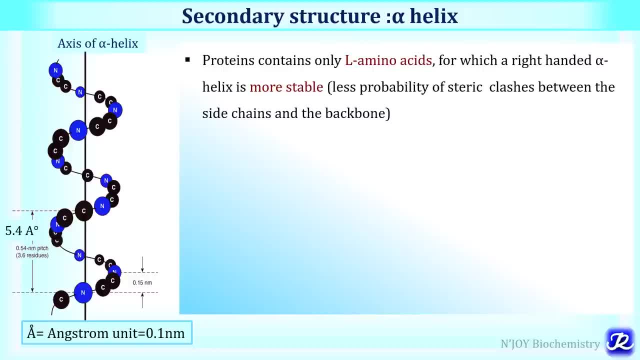 alpha helix is more stable and that's why in the protein only right-handed helix are present and why this alpha helix is more stable: because there are less probability of steric clashes between the side chains and the backbone. that's why The proteins have right-handed alpha helix and a complete turn of helix because of 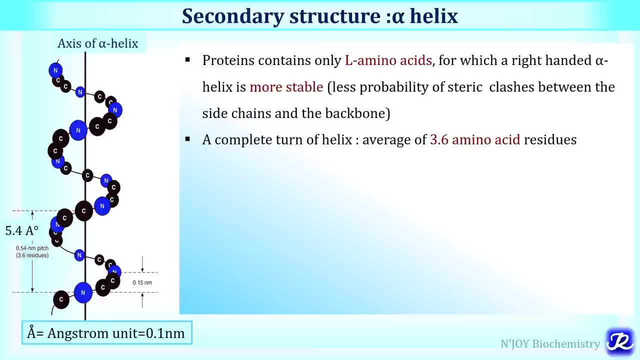 intramolecular hydrogen bonding, there is formation of. because of folding, there is formation of turns and each turn has average of 3.6 amino acid residues. and the distance- distance per turn- it is called as pitch- it is 0.54 nanometer or it is a 5.4 armstrong unit, because one 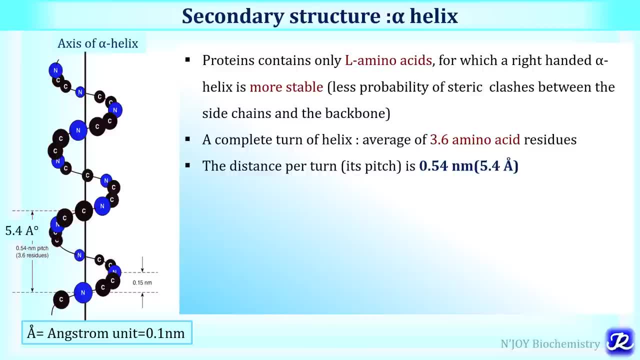 armstrong unit is a 5.4 armstrong unit. So it is a 5.4 armstrong unit because one armstrong unit is equal to 0.1 nanometer, So the distance per turn is 0.54 nanometer and the actual distance between: 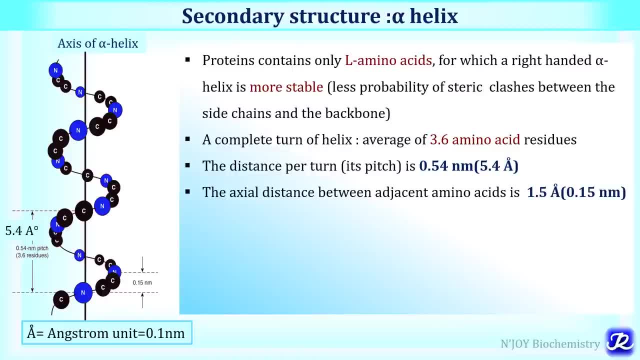 adjacent amino acids. so there is distance between each amino acid is 0.15 nanometer, which is 1.5 armstrong unit, and except for the first and last peptide bonds at both ends of the chain, all other groups take part in the hydrogen bonding. 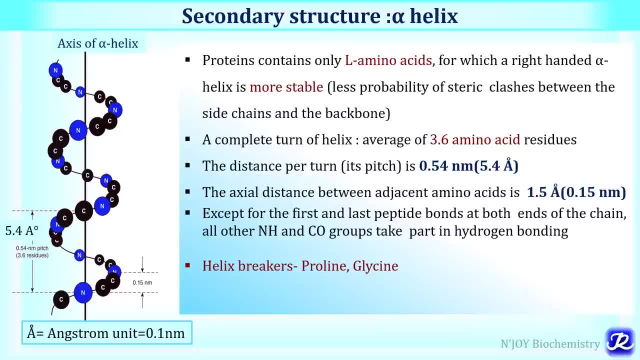 There are certain amino acids which do not participate in this alpha helical structure, and these are called as the helix breakers. proline and glycine. these are known as helix breakers And the examples of this secondary structure alpha helux, the fibrous proteins, are alpha carotene. 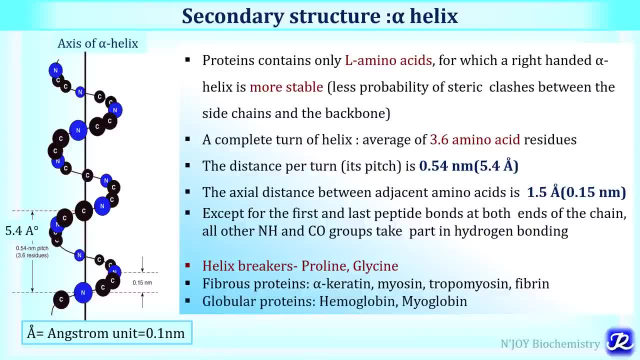 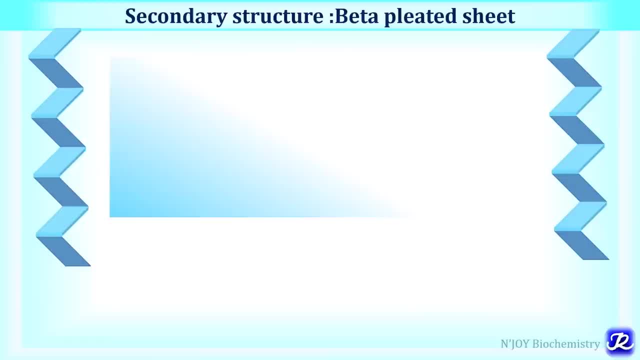 myosin, prop, only myosin, fibrin and the globular proteins like hemoglobin and myoglobin. they are made up of this alpha helical secondary structure. the second type of structure is called as beta plated sheet. it is called as beta because it is the second structure. 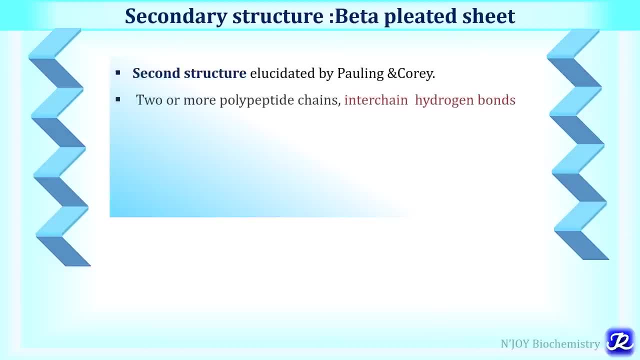 which was elucidated by the scientists Pauling and Corey, and in this structure, instead of one polypeptide chain, there are two or more polypeptide chains. and these chains are? they are linked by inter chain hydrogen bonds and this beta plated sheet. they are fully extended and that's why they. 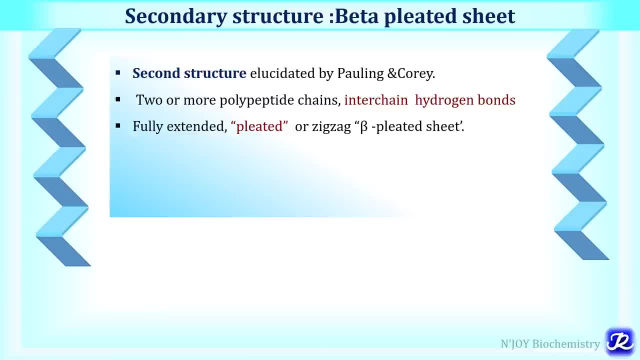 are called as plated or zigzag beta plated sheets. the axial distance between adjacent amino acids in beta plated sheet is 3.5 Armstrong unit, while in case of alpha helix the distance between adjacent amino acid was 1.5 Armstrong unit, but here the distance is 3.5 Armstrong unit. 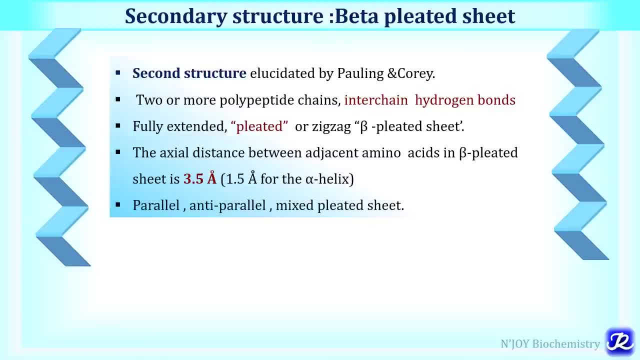 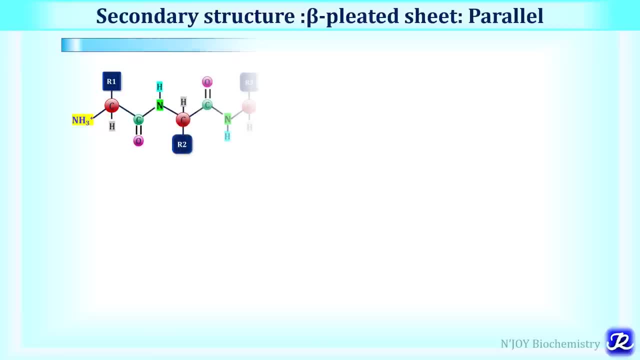 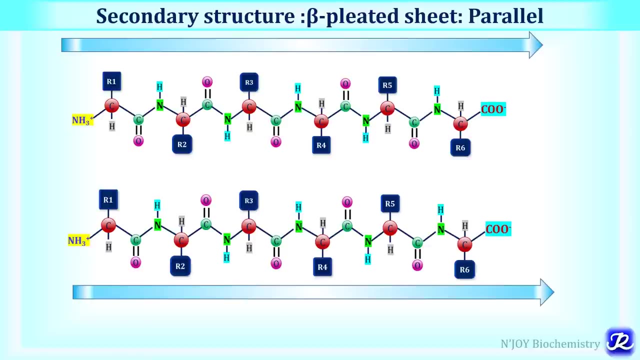 there can be parallel, anti-parallel and mixed plated sheets. in parallel beta plated sheet both the polypeptide chains. they are running in the same direction. so when both polypeptide chains are running in the same direction, they willヤ是這樣ly. 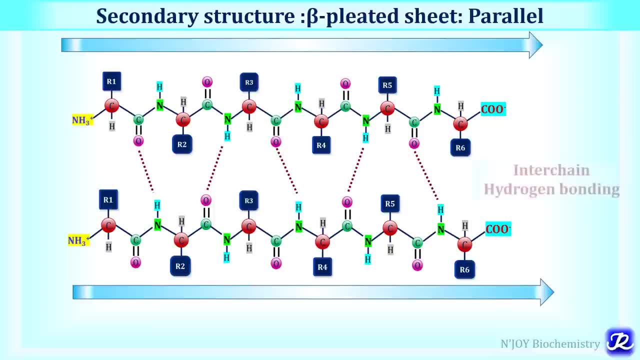 same direction. they are parallel to each other and hydrogen bonding is formed between these two polypeptide chain. it is called as parallel beta pleated sheet, and the example of parallel beta pleated sheet is flavodoxin. in the flavodoxin parallel beta pleated sheets are found. 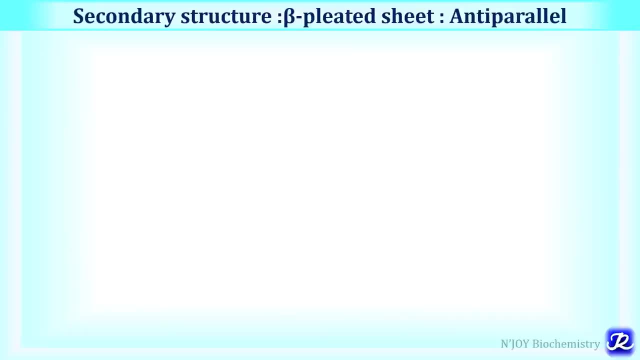 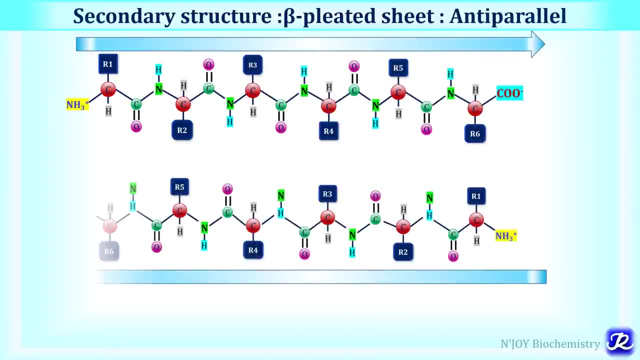 when two polypeptide chains are running in the opposite direction, they are called as anti-parallel beta pleated sheet. for example, this polypeptide chain is running from left to right and this second one is running from right to left, so they are anti-parallel to each other. and when there is 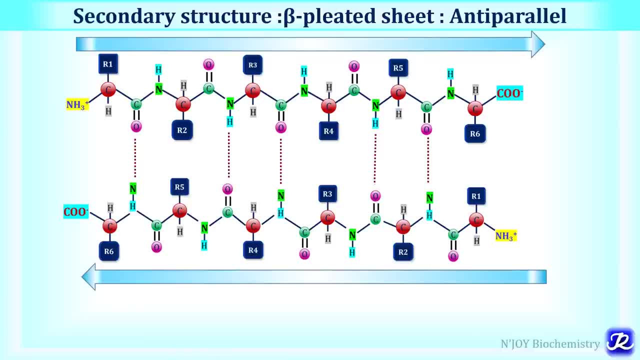 formation of inter-chain hydrogen bonding. it is called as anti-parallel beta pleated sheet and these anti-parallel beta pleated sheets are present in the silk fibroin and there are. there can be mixed beta pleated sheet where both parallel and anti-parallel beta sheets are present. 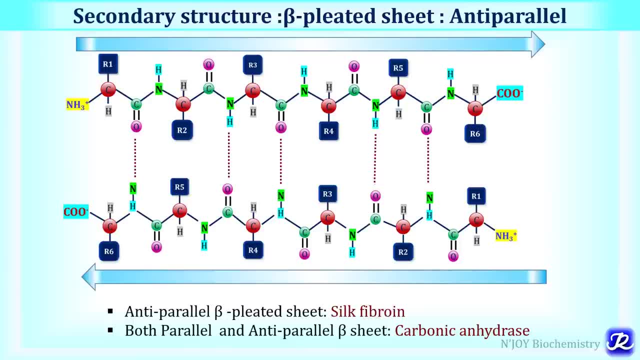 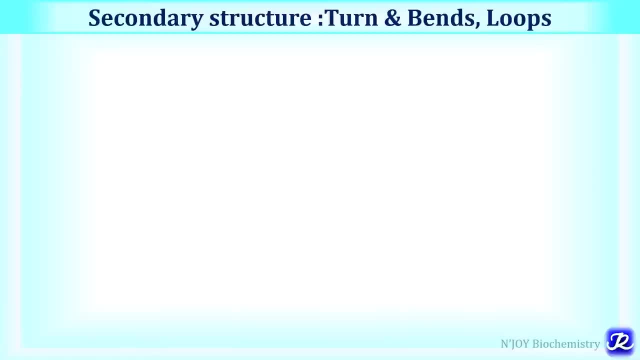 and both this parallel and anti-parallel beta sheets are present in carbonic anhydrase. other than alpha helix and beta pleated sheet, other secondary structures are turns and bends and loops. typical globular protein: it has half of the alpha helices and beta sheets and half 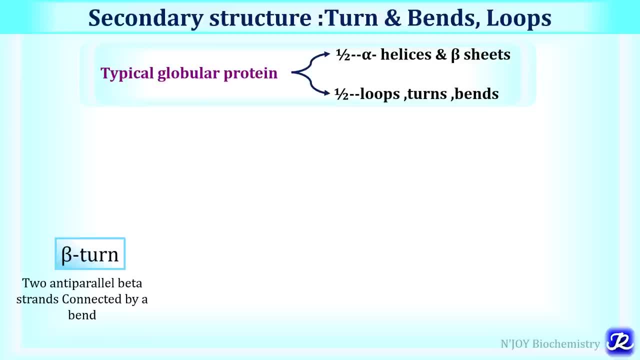 loops, turns and bends. so what is the beta turn turn when two anti-parallel beta strands. they are connected by a bend. it is called as beta turn. so here one polypeptide chain is running in the upward direction and other is the beta turn. so here one polypeptide chain is running in the upward direction and other is the. 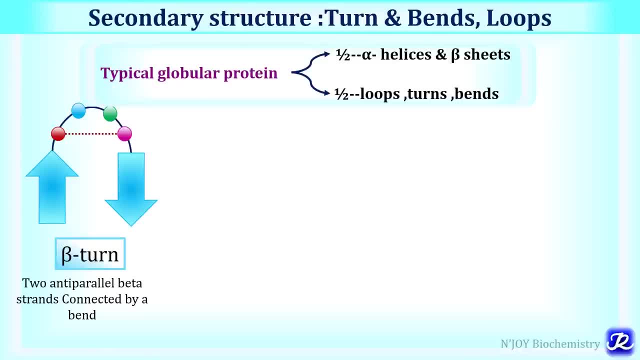 it is running in the opposite direction. so two polypeptide chains are anti-parallel to each other and both this polypeptide chain. they are connected by a band, so it is called a beta turn and this beta turn make polypeptide chain a compact molecule: glycine and proline residues. 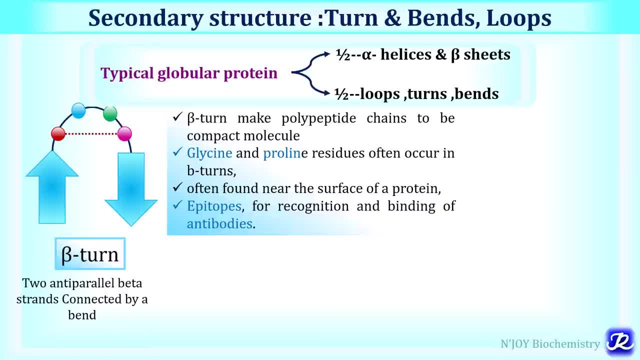 often occur in such beta turns, and these beta turns are often found near the surface of protein, for example epitopes, and these epitopes are useful for recognition and binding of antibodies. so this is the importance of beta turn in a protein structure. the other example of secondary 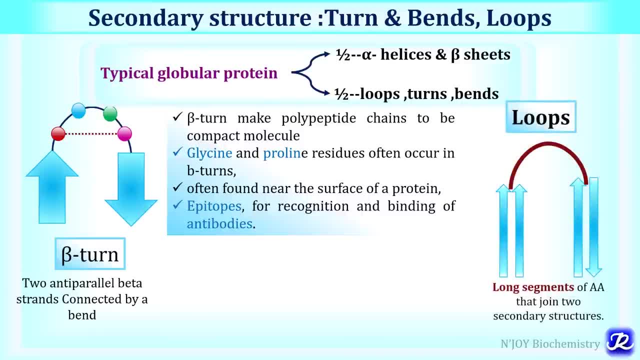 structure is loops. so loop is long segments of amino acids. that joins two secondary structure. it is called as loops. there is one more secondary structure called as triple helix. so in this triple helix three helices are present. so in this triple helix three helices are present. 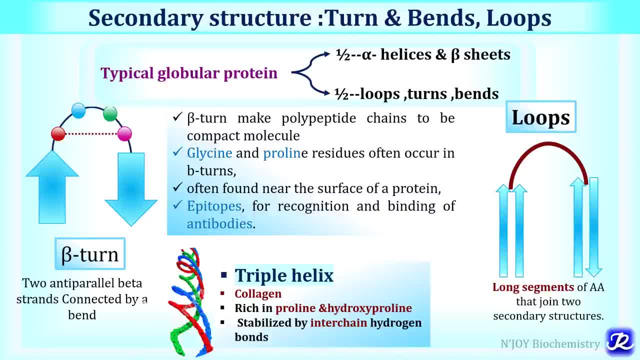 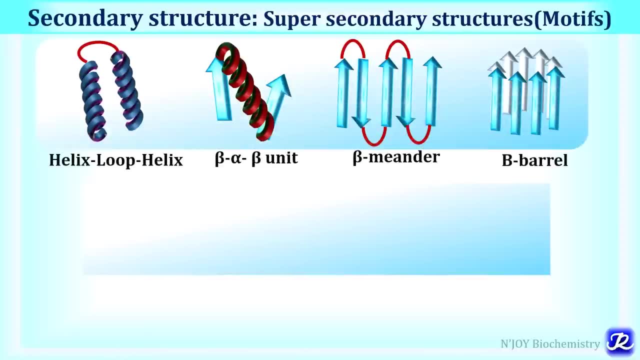 and in this triple helix, three helices are present And it is most commonly present in the collagen, which is rich in proline and hydroxyproline. and this triple helical structure, it is stabilized by inter-chain hydrogen bonds, Super secondary structures or various motifs. they are also example of secondary structures and various super secondary structures are helix, loop helix, where two helices or two helix are. they are connected by a loop. 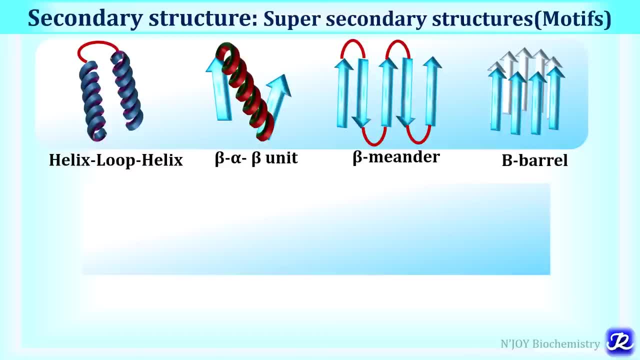 Beta, alpha beta subunit, where two beta plated sheets is connected by alpha helix, beta meander and beta barrel, So globular proteins. they are constructed by combining this secondary structural elements like alpha helices, beta sheets and various non-repetitive sequences. 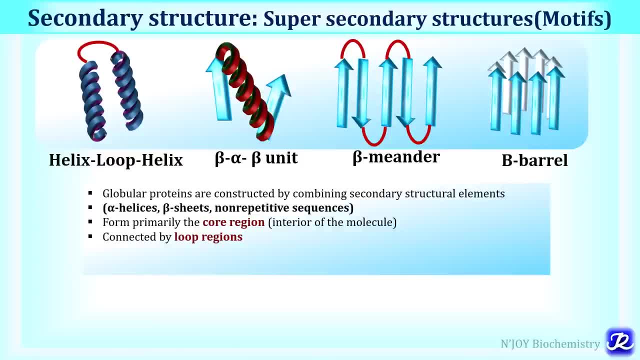 And they form primarily the core region, that is, the interior of molecule, which are connected by the loop region And they are produced by packing side chains from the Adjacent secondary structural elements close to each other. So these are the examples of super secondary structures: helix, loop, helix, beta alpha, beta unit, beta meander and beta barrel. 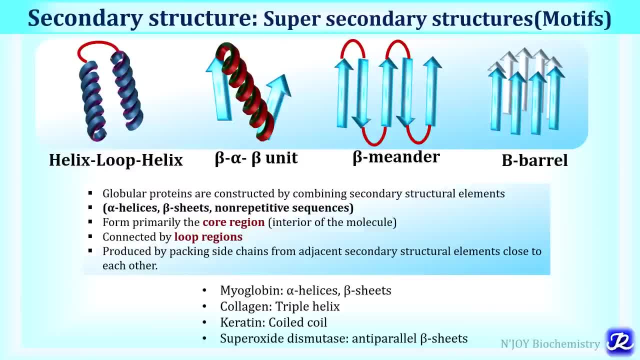 There are various structural motifs which are present in the proteins, like myoglobin. Myoglobin consists of both alpha helices and beta sheets. Collagen is made up of triple helix, Aritin has coiled coil and superoxide dismutase has anti-parallel beta sheets. 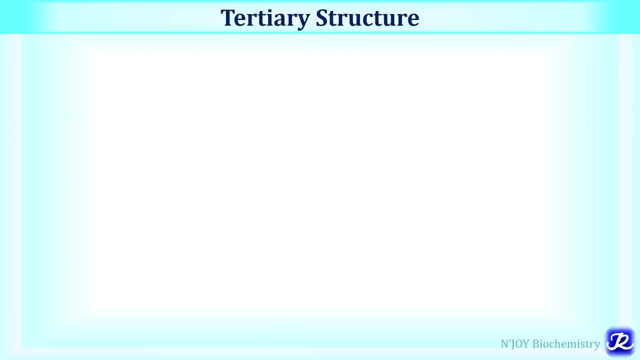 Coming to the tertiary structure, the peptide chain with its secondary structure may be further folded and twisted about itself, forming three-dimensional arrangement of the polypeptide chain And the three-dimensional folded, compact and biologically active conformation of a protein. it is referred as tertiary structure. 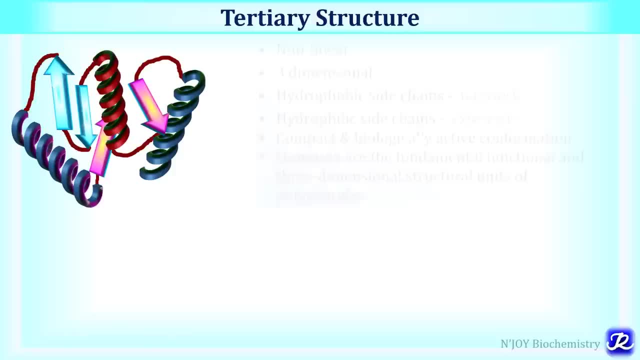 So this is a three-dimensional structure. tertiary structure is a three-dimensional structure. It is non-linear- hydrophobic side chains are present interiorly and hydrophilic side chains are present Exteriorly, and it is a compact and biologically active conformation and it has domains, and domains are the fundamental functional and three-dimensional structural unit of polypeptides. 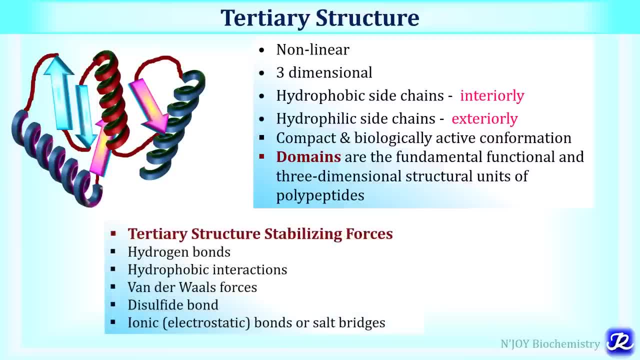 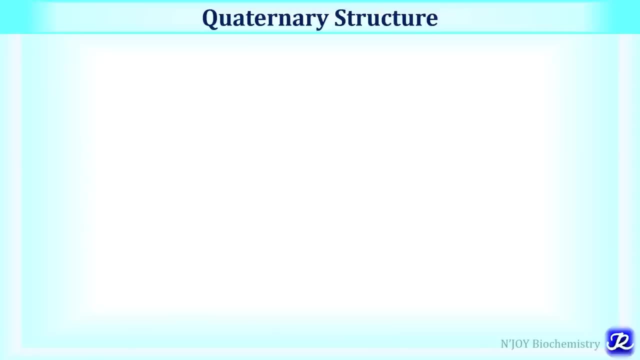 Now this tertiary structure is stabilized by various forces like hydrogen bonds, hydrophobic interactions, Winder-Wals forces, disulphide bond and electrostatic bonds or salt bridges. Coming to the fourth organizational structure, Organizational level of protein structure that is called as quaternary structure, 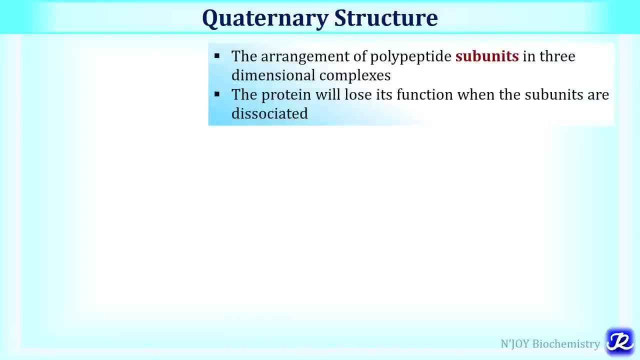 and here the arrangement of polypeptide subunits in three-dimensional complexes. so various subunits, they are arranged in a three-dimensional structure. The protein will lose its function when the subunits are dissociated. So all the polypeptide chains, they are integrated or they are arranged together. 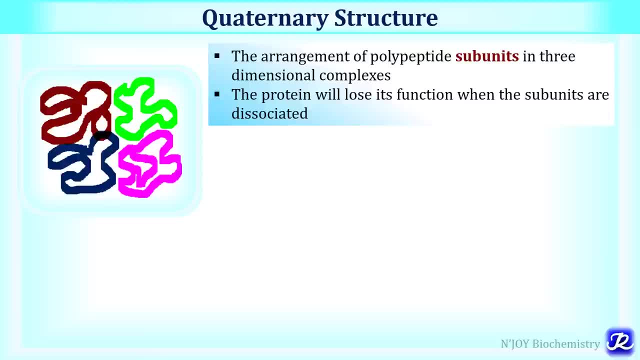 So different polypeptide subunits. they are arranged in a three-dimensional structure. It is called as quaternary structure structure, and this quaternary structure is stabilized by hydrophobic interactions, hydrogen bond, ionic bonds and van der Waals forces. The examples of this quaternary structure: 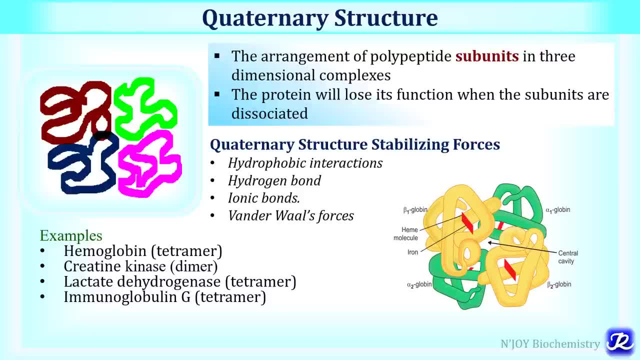 are hemoglobin. Hemoglobin is a tetramer. It is made up of four polypeptide units. Creatine kinase. it is a dimer. It is made up of two polypeptide units: Lactic dehydrogenase and immunoglobulin G. 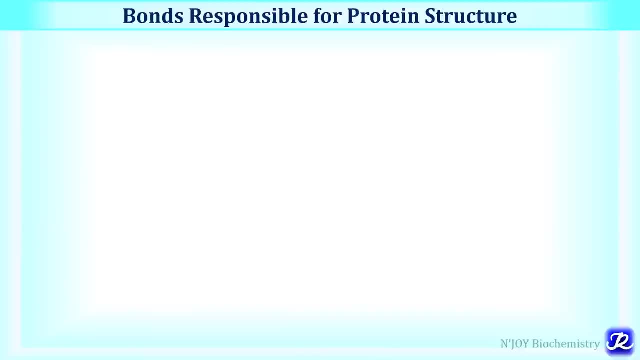 these are also tetramers. So far we have studied the four levels of structural organization of protein, that is, primary, secondary, tertiary and quaternary. Now we will study the bonds responsible for protein structure. There are two types of bonds: covalent bond and non-covalent. 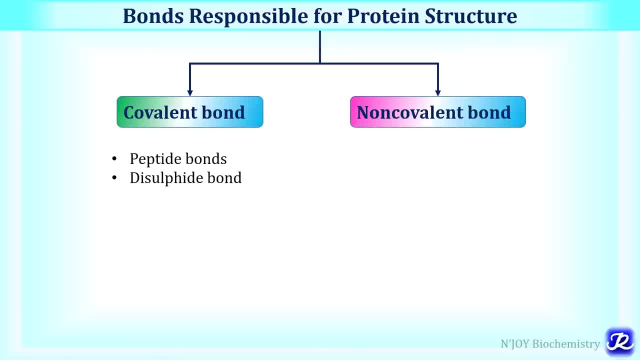 bond. The examples of covalent bonds are peptide bonds and disulfide bonds and hydrogen bond, hydrophobic interactions, electrostatic bonds, van der Waals interaction. These are the examples of covalent bonds. So far, we have studied the four levels of structural organization of protein. 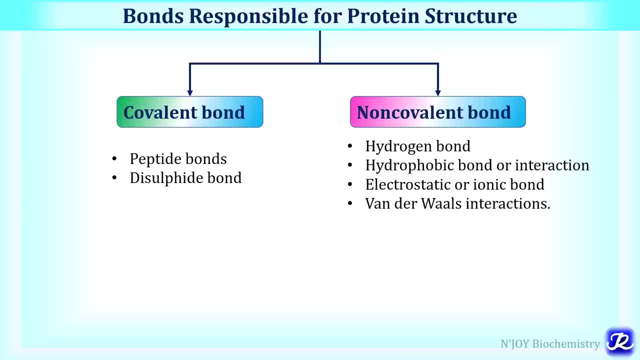 So proteins are nothing but linear polymers of L-alpha amino acid which are linked together by peptide bonds, and this peptide bond is a covalent bond. So this bond is formed by condensation of amino group of one amino acid with the carboxyl group of another amino acid, with a removal of. 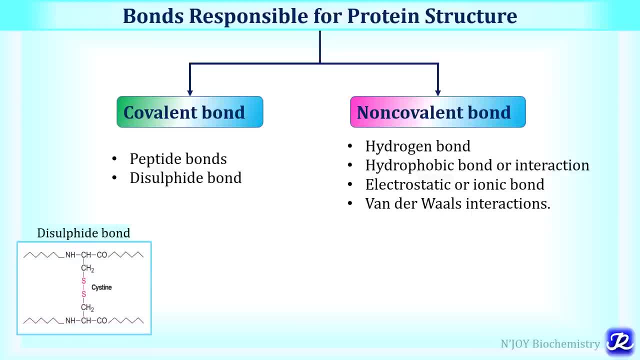 water molecule. Now the disulfide bond. This bond is formed between sulfhydryl group of side chain of cysteine residue. So this is disulfide bond. Now we will study the bonds, covalent bond and hydrogen bond. These are the examples of covalent. 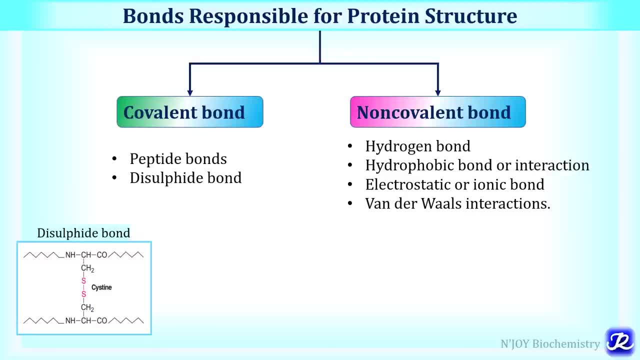 bonds. Now coming to the non-covalent bond. hydrogen bond, The hydrogen bond. it is formed between NH and CO groups of peptide bond by sharing single hydrogen and side chains of some amino acid can also form hydrogen bonds. Now hydrophobic bond or interaction. These bonds are: 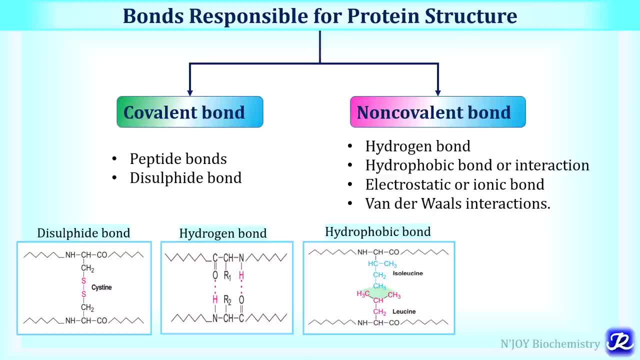 formed by interaction between non-polar hydrophobic R groups, that is, side chain of amino acids like alanine, valine, then leucine, isoleucine, methionine, phenylalanine and tryptophan, Then electrostatic or ionic bond. These are formed between oppositely charged groups, such as 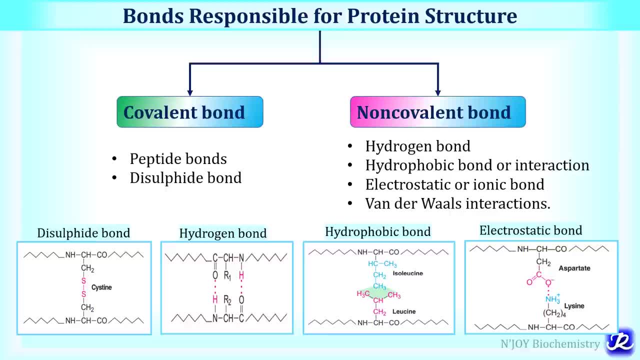 amino terminal and carboxyl terminal groups of the peptide and oppositely charged R groups of the polar amino acid residues And Van der Waal interactions. They include both an attractive and repulsive forces between both polar and non-polar side chains of amino acid residues. So these are 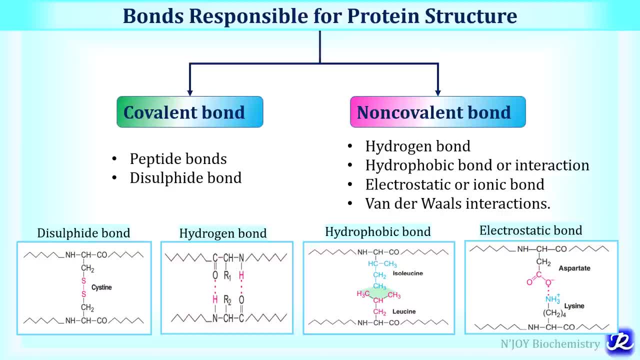 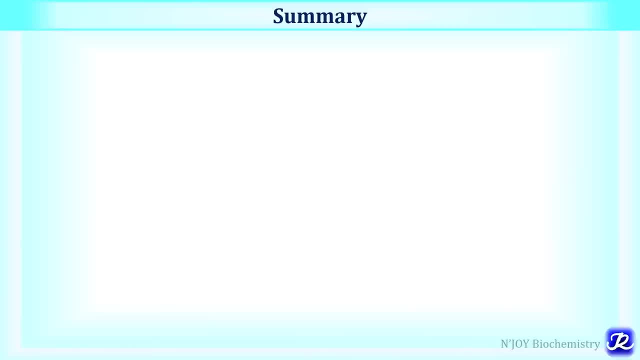 the different types of bonds which are responsible for variety of protein structures. So let's summarize the topic. There are four levels of organization of protein structure: Primary, secondary, tertiary and quaternary. And it is the result of assembly of different amino acids which are linked together by peptide linkages, Then folding of that primary structure. 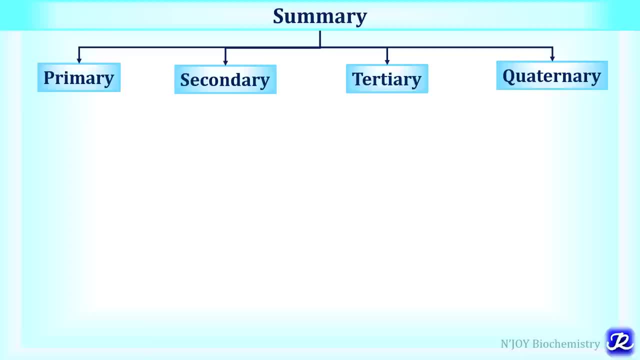 leads to secondary structure, Then three-dimensional structure leads to secondary structure, Then three-dimensional arrangement of secondary structure leads to formation of tertiary structure, And then three-dimensional arrangement of different polypeptide units. together it is called as quaternary structure, So primary structure. it is the sequence of amino acid which is linked by